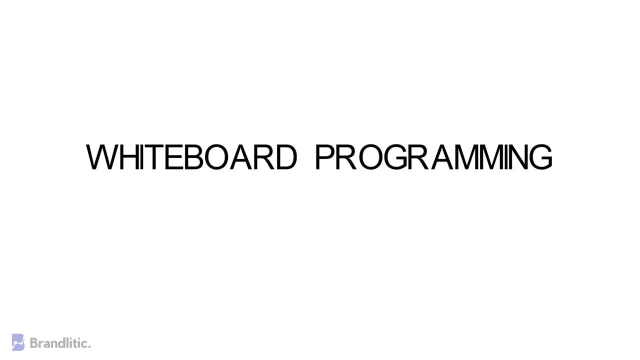 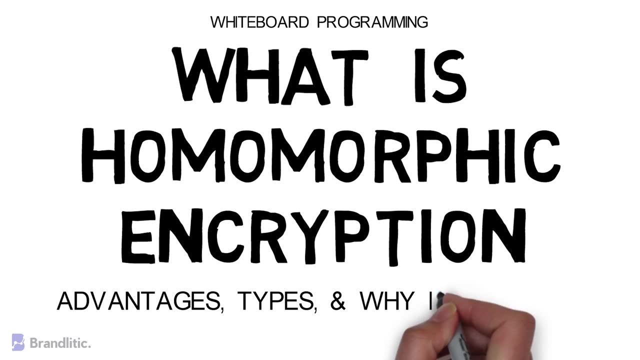 Welcome to whiteboard programming, where we simplify programming with easy to understand whiteboard videos, and today i'll be sharing with you what is homomorphic encryption, its advantages, why it should be employed, types of homomorphic encryption and a lot more. so let's get started. firstly, let's understand the meaning of the term homomorphic. it is fundamentally based out in: 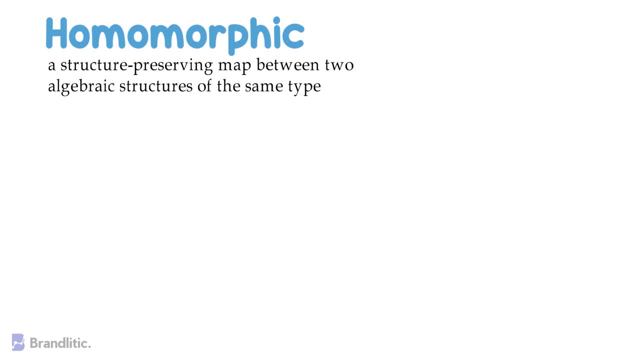 algebra and means a structure preserving map between two algebraic structures of the same type, that is, it can be two groups, two rings or even two vector spaces. so, similarly, when someone asks what is homomorphic encryption, we can simply understand it as a form of encryption that 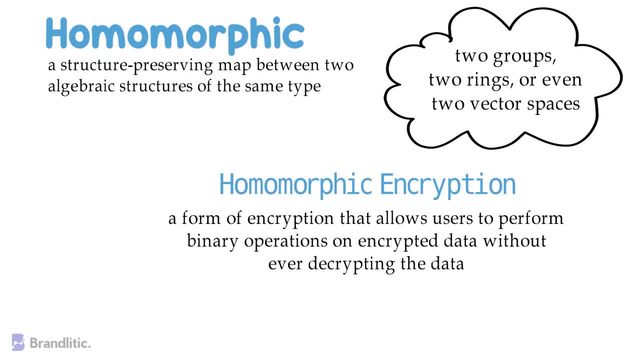 allows users to perform binary operations on encrypted data without ever decrypting the data first, and it is because of this encryption only that we are able to perform binary operations on encrypted data without ever decrypting the data first, and it is because of this encryption only that we are 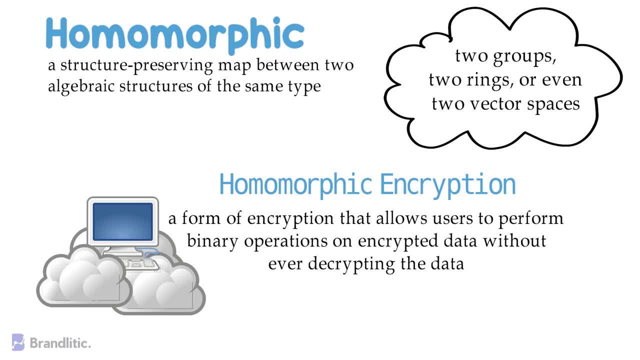 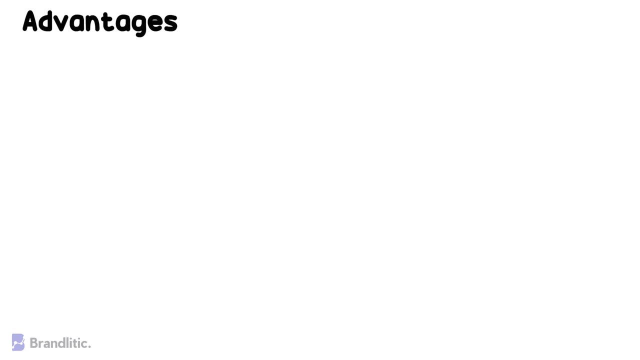 able to encrypt and outsource information to a cloud service or environments for processing without giving any third party access to our raw data. cool, right now. let's look into some of the advantages of homomorphic encryption quickly. well, the biggest one being that it's heavily privacy friendly if we employ it and also do. 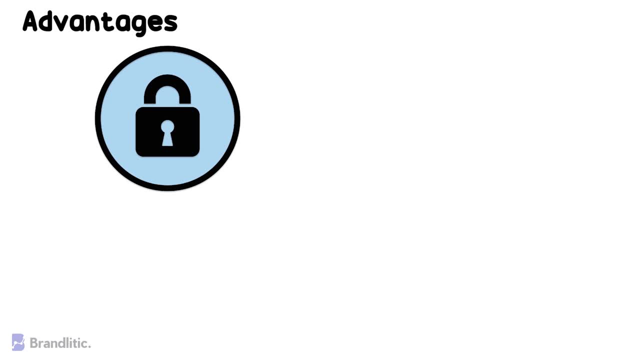 note that in today's world, if we want to perform computations on encrypted data, such as mathematical operations, we have to decrypt the data first and then only we have to make our necessity computations and finally encrypt the data again in order to send it back. but what happens when the encrypted 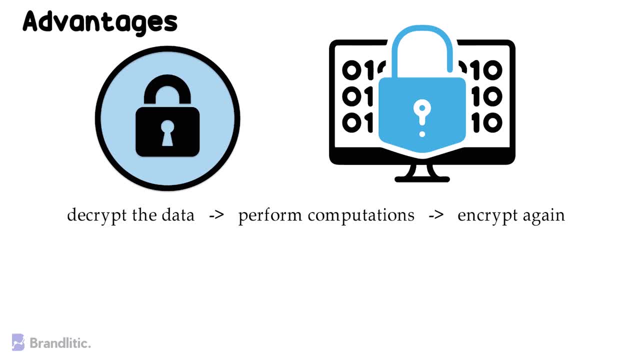 data is very sensitive and we don't want other services to have access to them. here is where homomorphic encryption comes into play. a more practical example would be a system or a service that processes medical information in order to diagnose if a patient is suffering from a disease. 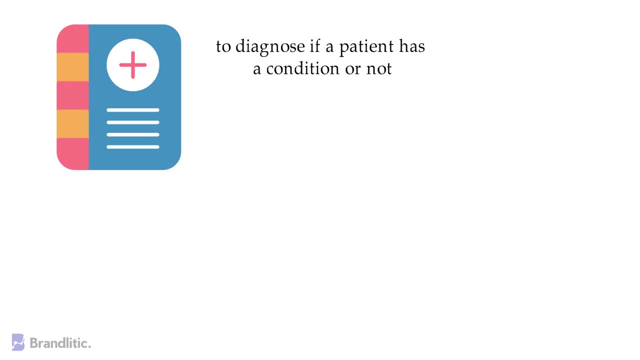 if a patient has a condition or not. the data we'd be sharing probably includes very sensitive information about patients medical history, so this is something we want to ensure won't be accessible to someone else apart from the authorized personnel now here. by using homomorphic encryption, the system or service can process the required computation on the encrypted. 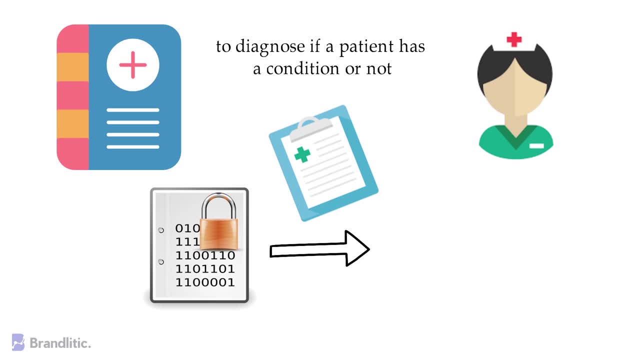 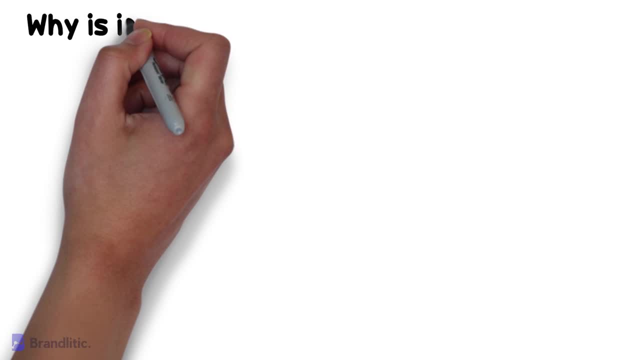 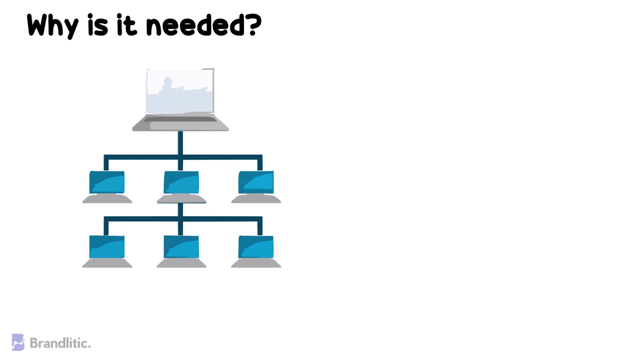 data, returning the result of the diagnosis, without knowing which information is being processed. if you are still confused, let me try and explain again on why is homomorphic encryption needed in the first place? well, by sharing sensitive information through any platform, one can easily give away their privacy. on the other hand, being able to modify and perform, 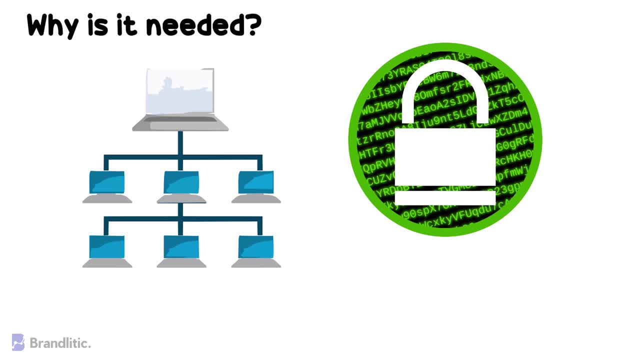 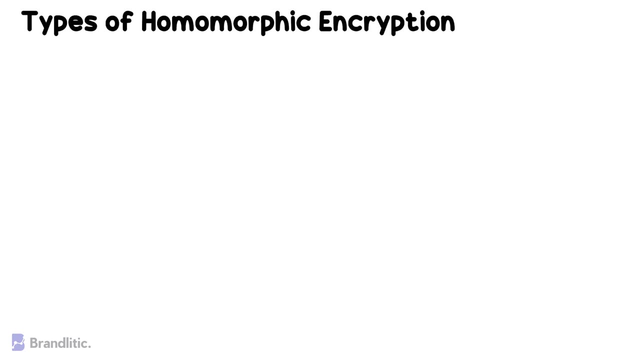 operations on data while they are still encrypted ensures the privacy of the data, which, in today's digital world, is highly important. next, let's look into the different types of homomorphic encryption. the most common types of homomorphic encryption include number one: partially homomorphic encryption, or phe, which allows for only one operation to be performed. 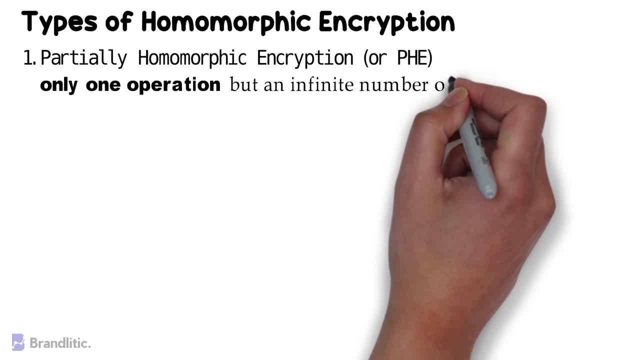 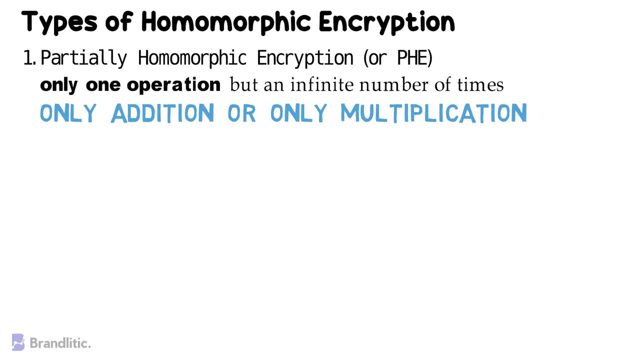 on the ciphertext, but an infinite number of times. now this operation can only be of addition or only multiplication in its nature. further, these are a lot easier to design and are very powerful in applications that use one arithmetic operation. number two, somewhat homomorphic encryption, or she, which allows both addition and multiplication to be performed, but for a 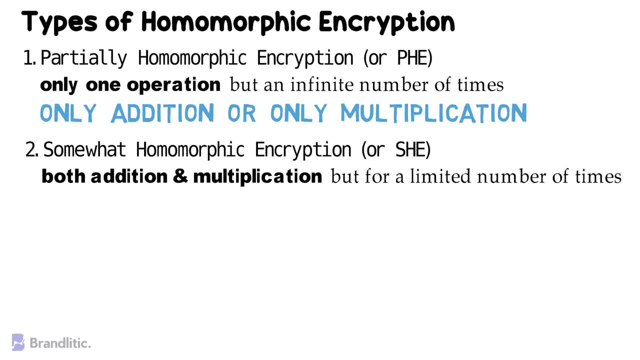 limited number of times and this limitation is evaluated to a certain depth in the circuit logic. number three: fully homomorphic encryption, or fhe, which allows both addition and multiplication to be on the ciphertext and an infinite number of times, and it also supports arbitrary computations on the encrypted data. 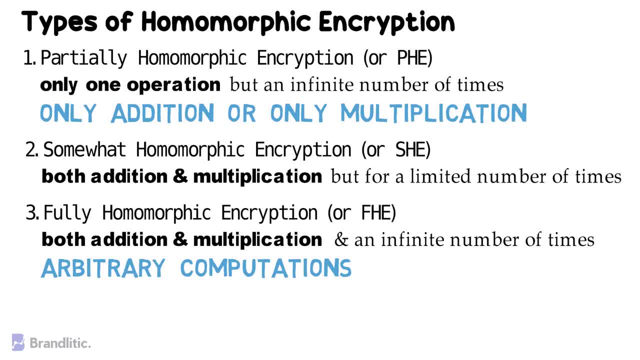 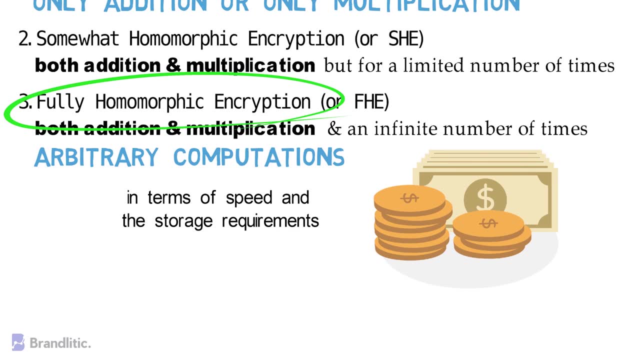 Now you might be thinking, knowing them all, that FHE or Fully Homomorphic Encryption is the best, but not exactly. The major problem with Fully Homomorphic Encryption is the cost efficiency, both in terms of speed and storage requirements, compared to plain text operations, which is something businesses. 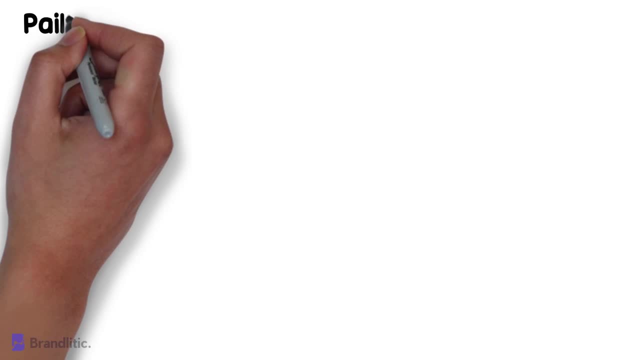 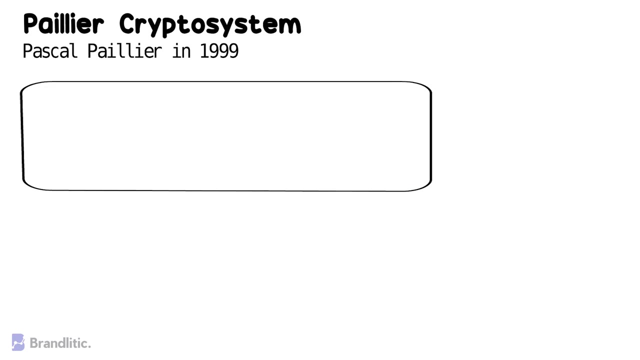 do care about. Next, let's look into the Paylier Cryptosystem, which was invented by Pascal Paylier in 1999.. The Paylier cryptosystem, inherently, is a partial homomorphic encryption or PHT scheme that works as additive, homomorphic in nature.